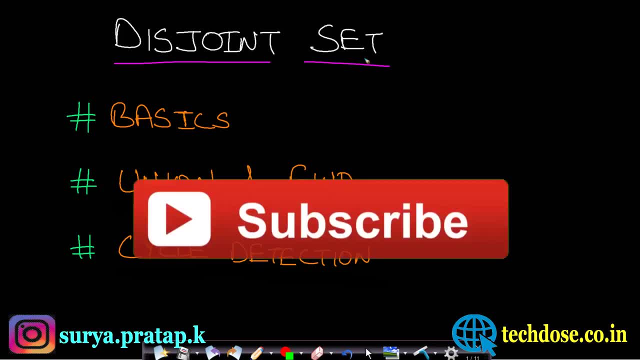 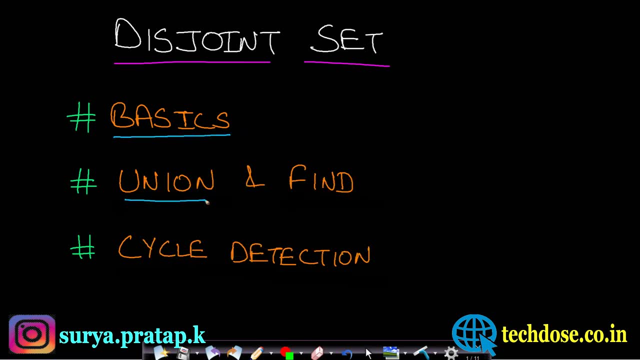 hello guys, welcome back to techdos. and in this video we will see the disjoint set data structure and in this video i will be just speaking about the basics of disjoint sets. i will show you two operations, which is the union, and find operations in disjoint set, and i will also show you a basic. 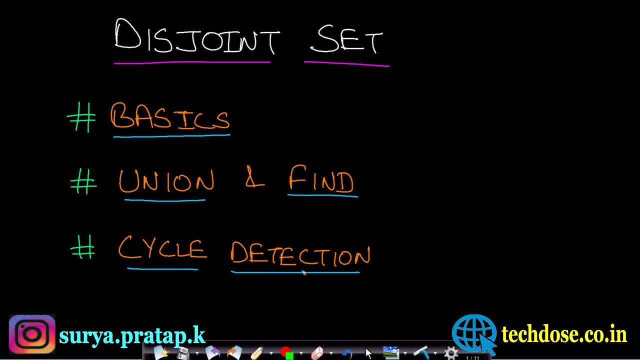 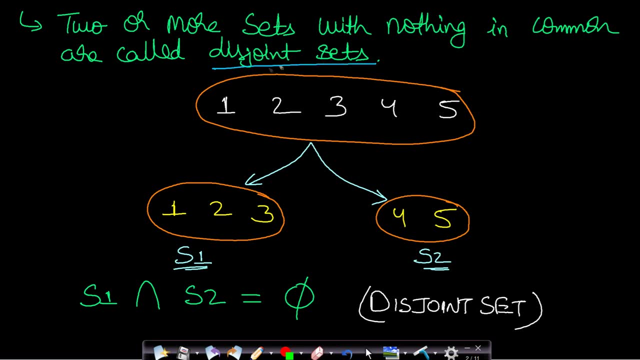 example, which is cycle detection in an undirected graph. so let us get started. two or more sets with nothing in common are called disjoint sets. this you must have figured out by the name itself. let us say you are having five elements- 1, 2, 3, 4 and 5- and let's say you divided them into two. 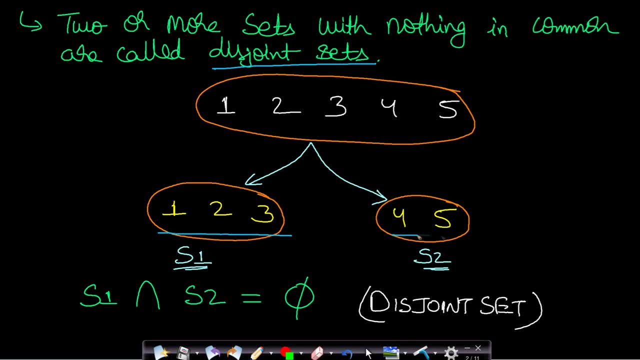 sets. set 1 is having elements 1, 2, 3 and set 2 is having elements 4 and 5, then you can see that there are no elements in common between these two sets. so if you take intersection between set 1 and set 2, then you will not get anything. then you can say that this set 1 and set 2 are disjoint sets. 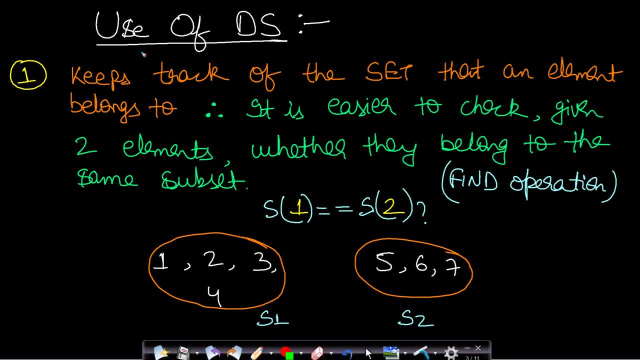 they do not have anything in common. now, what is the use of disjoint set? well, we have two popular uses. the first one is it keeps track of the set that an element belongs to. therefore, it is easier to check, given two elements, whether they belong to the same subset or not. 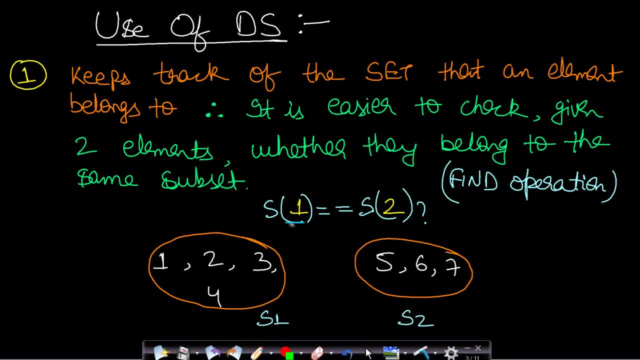 so in this case, let us assume that we want to find if this element 1 and this element 2 belongs to the same set or not. so how do we find it? we can use the disjoint set in order to find it if 1 belongs to the set to which this 2 also belongs. in this case, you can see that 1 and 2. 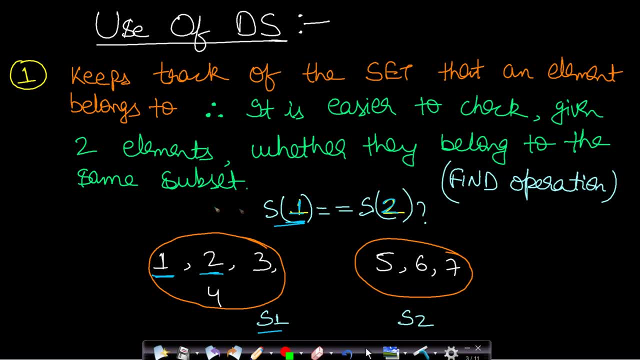 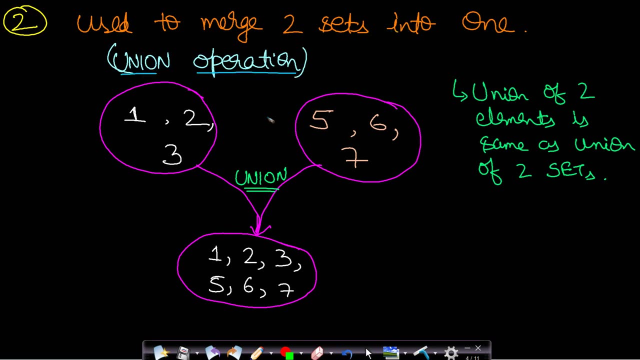 belongs to the same set, which is s1. therefore this will return true. this is nothing but the find operation in the disjoint set, which i will show you later in this video. now the second use is it is used to merge two sets into one. so this is nothing but union operation. you must be familiar. 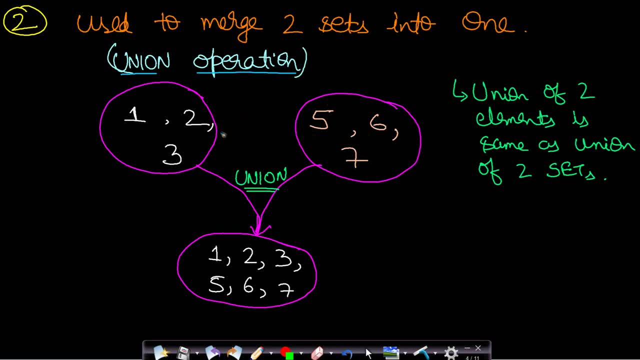 with this term from your set theory concepts as well. but in this case union of two elements is the same as union of two sets. so if i say that i will take union of this 2 and the 6, then this will be same as taking union of the set s1 and this set as to okay and after taking the union, 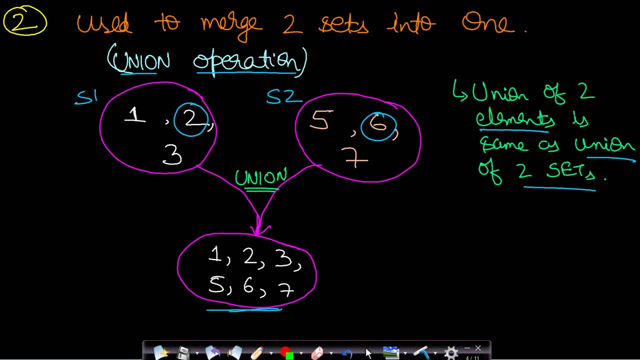 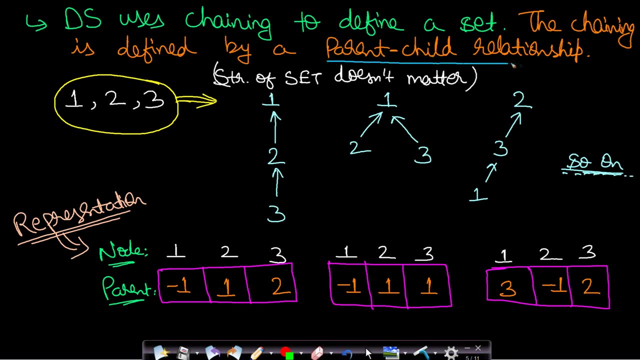 this will be the result. this is the second popular operation on disjoint set. now the disjoint said use is chaining to define a set. the chaining is defined by a parent-child relationship, so this is a hierarchical relationship. in this case, if your set is having three elements, let's say 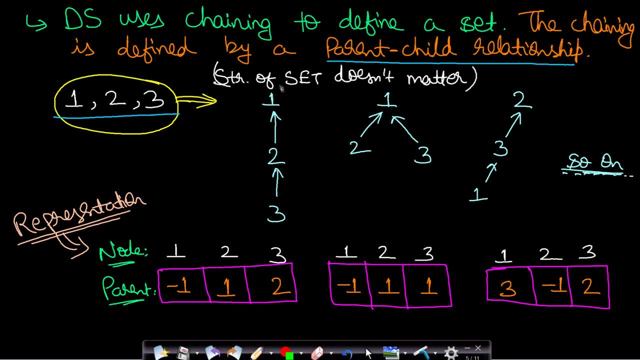 one, two, three, four and so on. so this set now cannot be chained and in this analysis, perhaps whine and 3, then you can represent it like a tree diagram, okay, and whatever elements are present in a tree will all belong to the same set. so you must be knowing that in a tree you have a root. 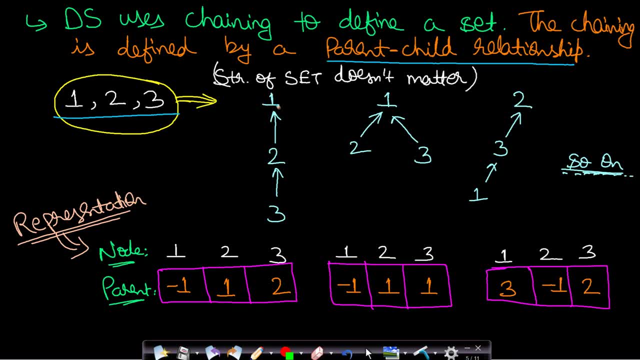 and there is only one root in a tree. okay, there can be any number of leaves, any number of internal nodes, but there will only be a single root for a entire tree. so in this case, let us say: you want to represent this 1, 2, 3 as this structure. in this case, what we have defined is: 2 is the parent of. 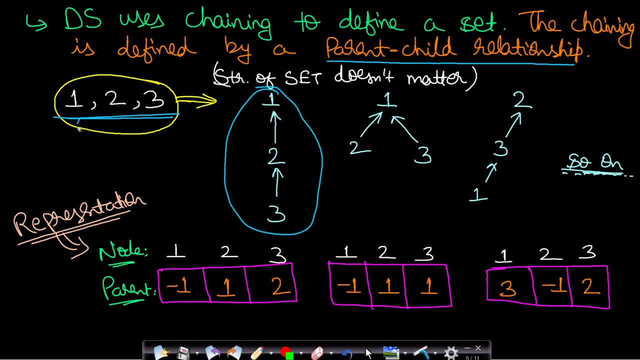 3 and 1 is the parent of 2. now, if you are given the query, let's say, if you want to find whether 1 and 2 belong to the same set or not, then what you can do is you can find the absolute parent. 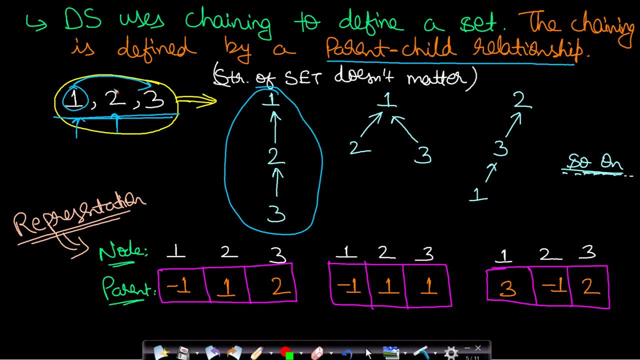 that is the root of the tree to which this 1 belongs and the root of this tree to which this 2 belongs. so, root of 1, that is, the absolute root of this 1, will be 3 and absolute root of this 2 will also be 3. so, since these two elements are having the same root, therefore, 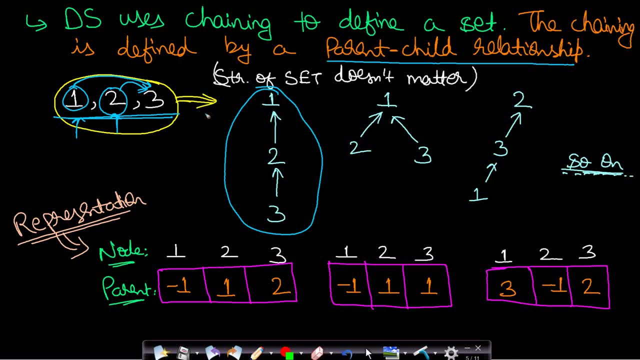 they will be belonging to the same set. this is the logic. okay, so you might be representing it by using different structures, but the structure of the tree actually does not matter. it just matters for your optimization purposes. the main thing which matters is inside a tree, all the 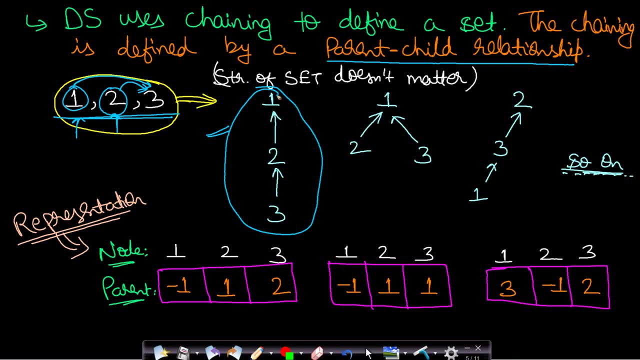 element will belong to the same set, and you already know that there will be only one single absolute root. okay, okay. so whatever structure you take, there will be only a single absolute root. so this is a second structure. in this case, if you want to find if one and two belong to the same set or not, then you 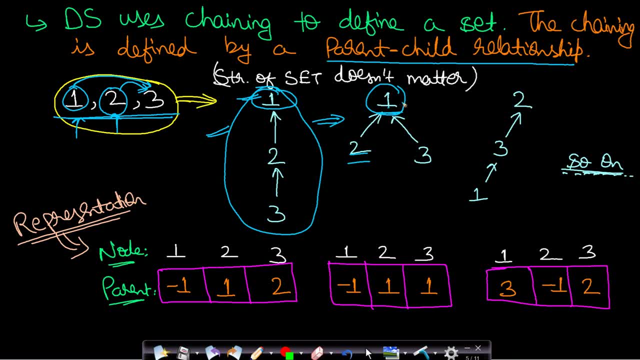 will find the absolute root of this one and two. for this one, the absolute root will be one. for this two absolute root will be one itself. therefore, since they both are having same absolute root, therefore they will both be belonging to the same set and the same logic goes. okay, so there can be. 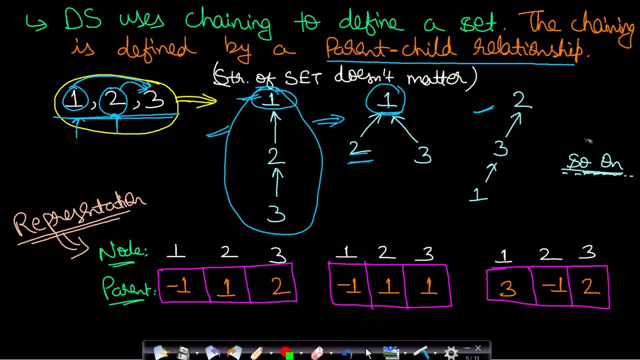 many more representations, but the structure will not really matter. it just matters for the purpose of optimization. now, how do you represent this tree structure? actually, that can be represented by using a simple array. okay, so let us assume that our elements are one, two, three. now how do you represent? 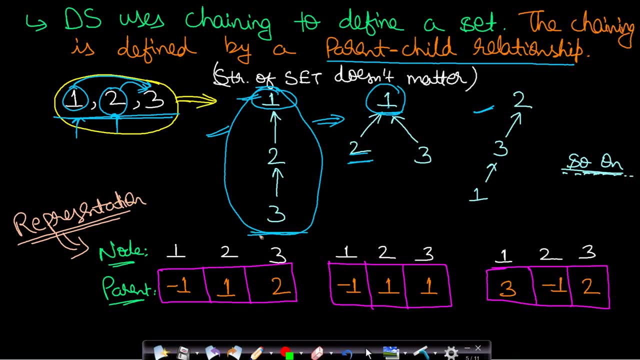 it by using an array. so if you want to represent, let's say, this first structure, then you will take an array and you will have indices. so the indices of an array will be assumed to be the node. so in this case our node values are one, two and three. so indices one, two and three will act as the node and whatever. 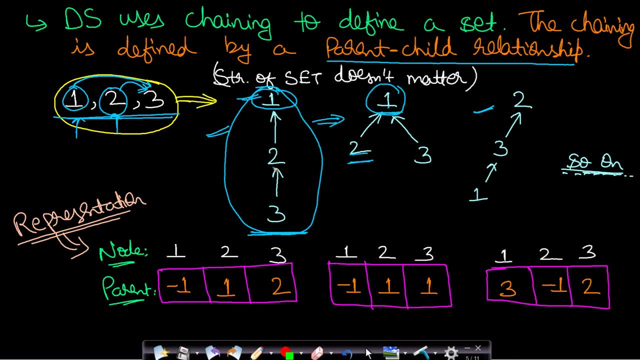 values they store will be nothing but the parent values to which they are pointing to. okay, so in this structure you can see that parent of three is two, therefore three. index three will be storing value two. now the parent of two is one, therefore index two will be storing value one and parent of. 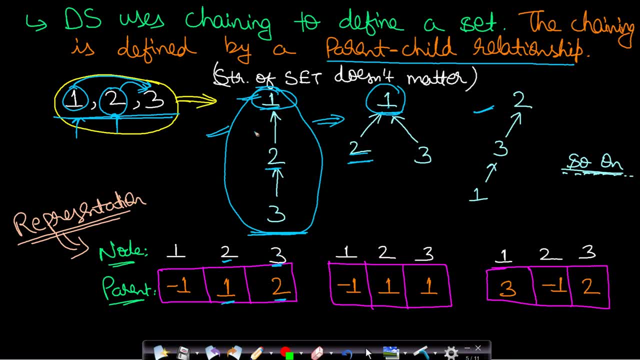 one is one itself. there is no parent of one. okay, so for this case, you will be storing minus one. now for the second structure. you can see that parent of three is one, so index three will be having value one. parent of two is one. therefore, index two will be having. 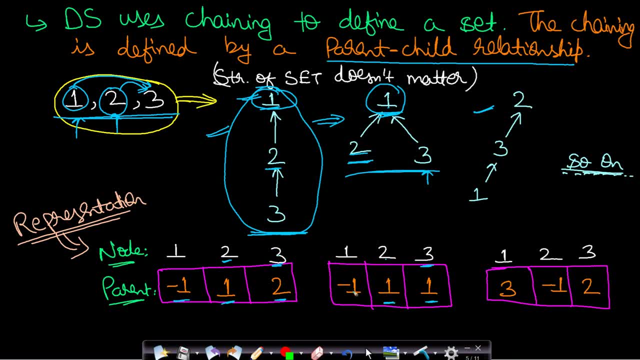 value one and parent of one is nothing, so this will be having value minus one, because this is the absolute root. okay, in the third structure you can see that parent of one is three, so index one will be storing value three. parent of three is two, so index three will be storing value two. 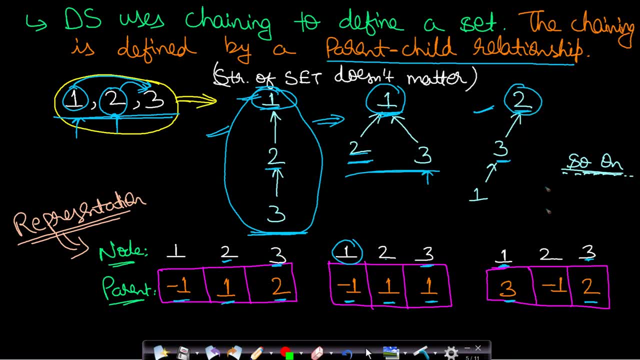 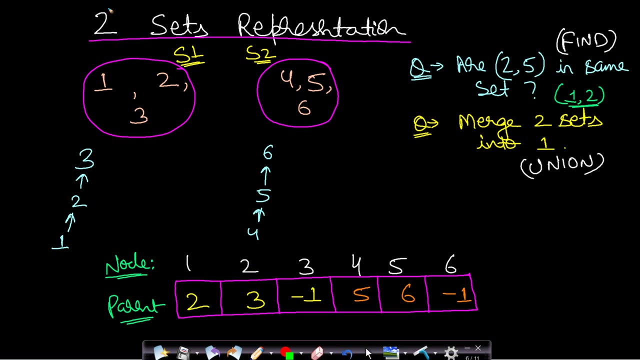 now parent of two is nothing. this is the absolute root. so this will be having value minus one. i hope you understood the representation of this structure in the form of an array. now, having understood this, how do we represent multiple sets using the array? so in this case, i will just represent: 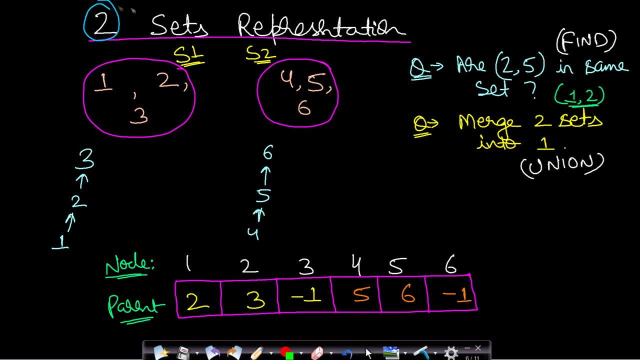 two sets using an array. you can represent more than two sets as well using the same array. okay, so let us assume that we have this set one as one, two, three set, two as four, five and six. now one simple structure can be a skewed tree where we assume that three is the absolute root. 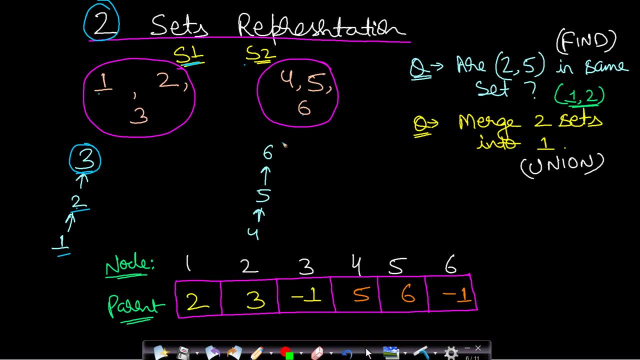 and three is the parent of two. two is the parent of one. similarly, we can assume that six is the parent of five. five is the parent of four. okay, now, in the representation i have already told you that the index values will act as the node values and whatever they store in the array, 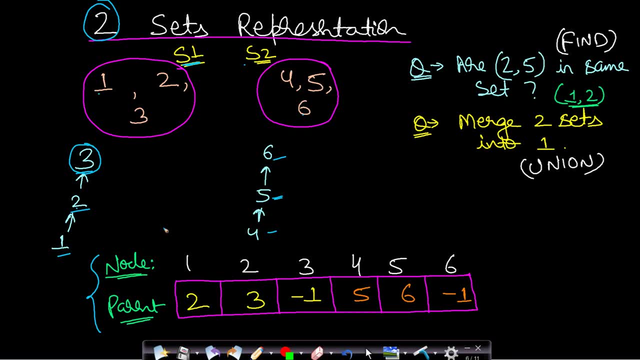 element will be nothing but the value of the parent node to which they are pointing to. so if we have set one structure, then one is pointing to two. this means that one is the child of two, okay, now two is pointing to three. that is, two is the child of three. now three is not pointing. 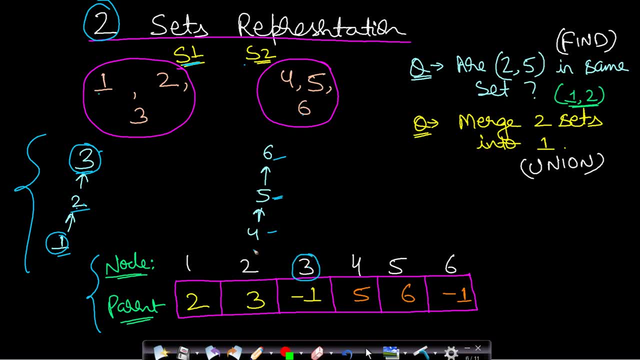 anywhere, therefore, three must be absolute root of its tree. okay, so in this structure, three is the absolute root. in the second structure, you can see that parent of four is five, so four will be pointing to five. parent of five is six, so five will be pointing to six. 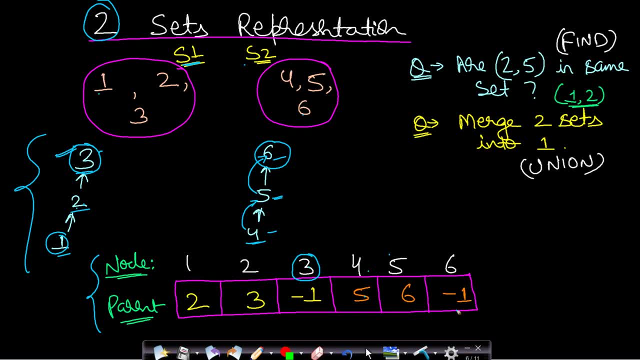 parent of six is nothing. this is absolute root. therefore, this will be minus one. okay now, these two sets are represented by using array. now, what are the operations which we can be required to find? there are two operations: one is find and another one is union. so what is the find operation? 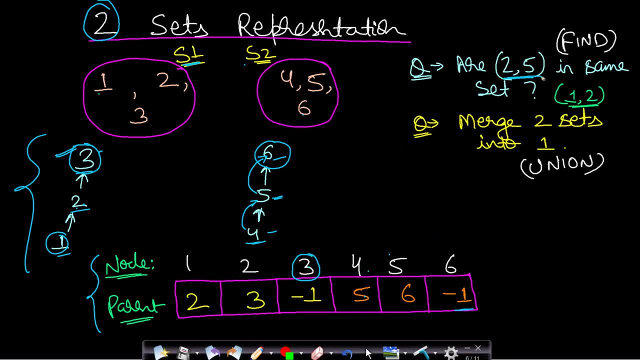 let us assume that you want to find whether two comma five, that is, two and five, belongs to the same set or not. so how do you find it? you will find the absolute root of this two, absolute root of this five, as i have already explained you. so if the absolute root of two, 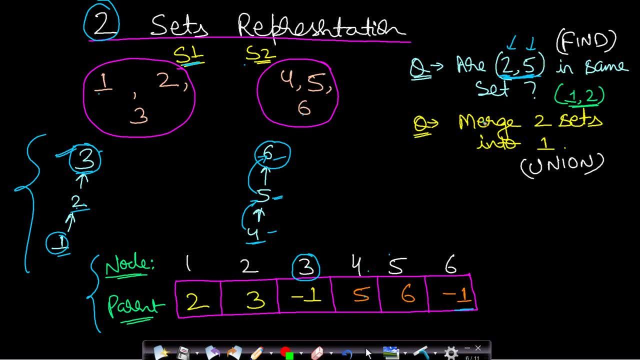 and absolute root of five are equal, then they will belong to the same set. in this case, if you go to this two, then it is pointing to three, so you will go to three. now for this three it is pointing to minus one. this means that this three is the absolute root, so absolute root of two will 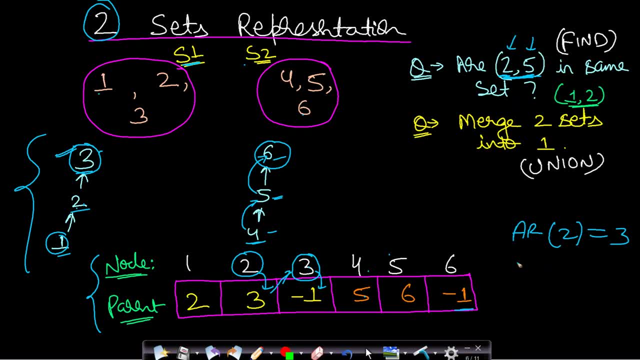 be equals to three. okay, now, similarly, you will find the absolute root of five: 5. so you will start with this value: 5. 5 is pointing to 6. you go to this 6. 6 is pointing to minus 1. so absolute root of 5 is nothing but 6. now you can see that absolute root of 2 and 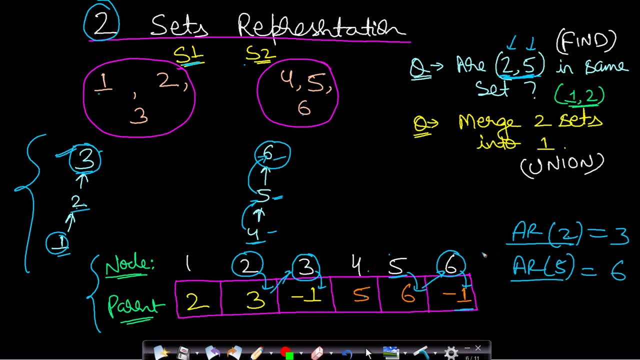 absolute root of 5 are not equal. therefore they must be present in different set. so in this way, you can find if two elements are present in the same set or not. this is nothing but the find operation, and similarly, if you are required to merge these two elements, that is, take union of. 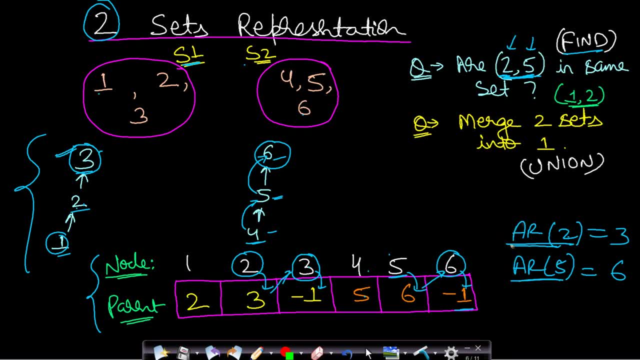 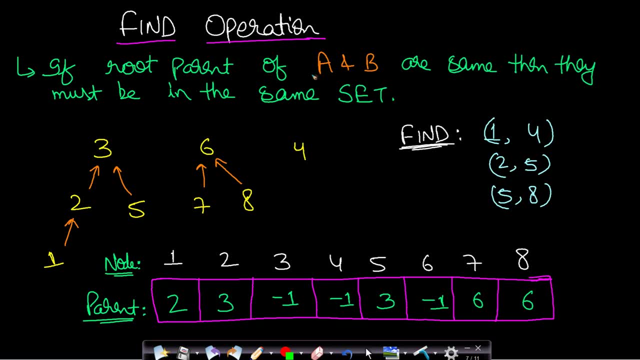 these two elements or these two sets to which these elements belong to, then that will be nothing but the union operation. so let us first see the find operation. if root parent of a and b are same, then they must be in the same set, otherwise they will be in the different set. so let us take three. 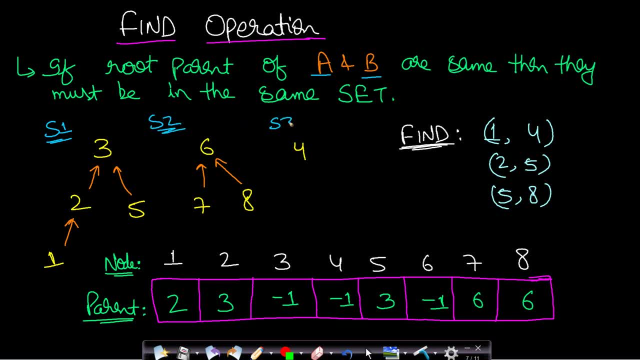 sets: this is set 1, this is set 2 and this is set 3, having just a single element: 4. so this is the array representation. the indices are representing the node values and the parent to which these indices are pointing to are stored in the array values. okay, so in this case we have 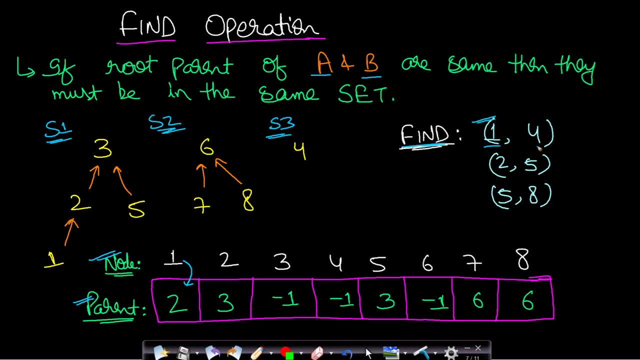 three find queries. so first find query is to find whether 1 and 4 belongs to the same set or not. so we will find the absolute root of 1. so we will start from 1. 1 is pointing to 2. we will go to 2. 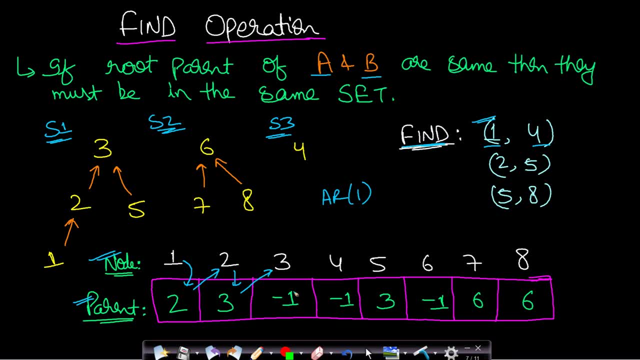 2 is pointing to 3, we will go to 3. so 3 is having value minus 1. so 3 will be absolute root and you will find absolute root of 1 will be equals to 3. okay now. similarly, we will find absolute root of 4. 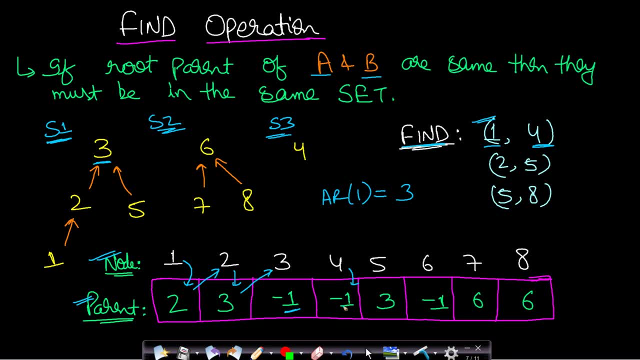 so we will go to this 4 now. for this 4 it is storing value minus 1, so absolute root of 4 will be equals to 4 itself. okay, so they both are having different absolute values. therefore they must be present in a different set. okay, so you will say you will return false. okay, so we will. 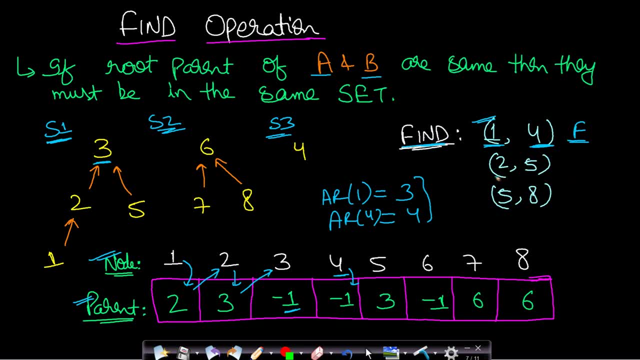 be returning true, if they belong to the same set. now for this second query, we will find absolute root of 3. we need to find whether 2 and 5 belong to the same set. we will now again start from this: 2. okay, so the absolute root of 2. we need to find it. it will be equals to 3, as i have already found for 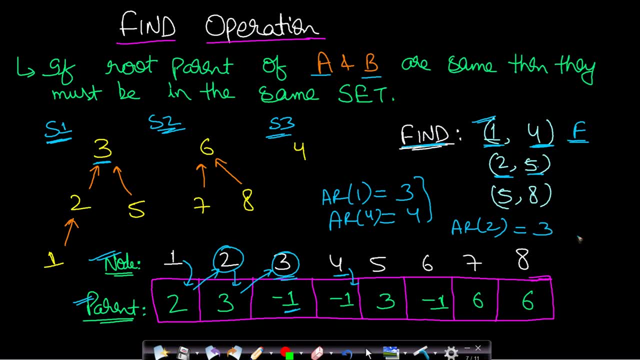 1, it will be 3. for 2, it will also be 3. so this is 3, absolute root of 5. this will be what for 5. we will start here. 5 is pointing to 3. we will go to this point 3. now 3 is pointing to minus 1. therefore, 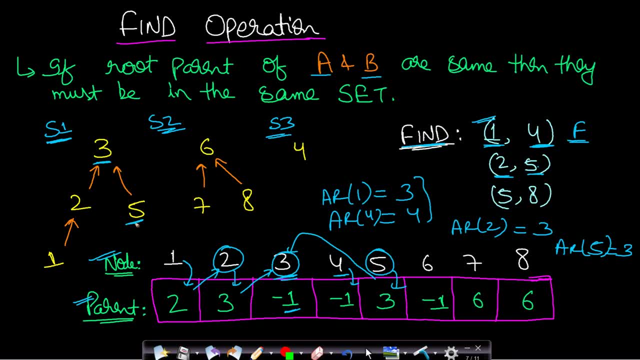 3 is the absolute root of 3, so we will start from this. 2. okay, so the absolute root of 3. we will go to absolute root of 5. you can see that in the diagram, 5 is pointing to 3. okay, so 3 is the. 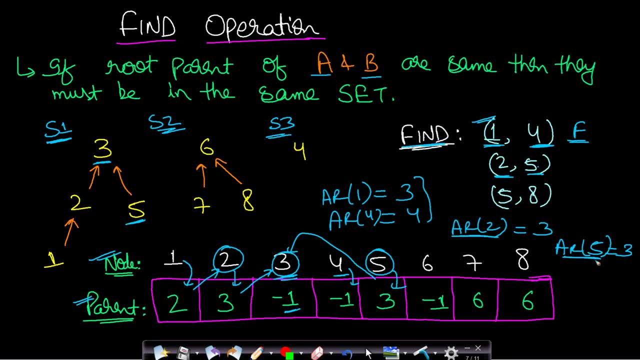 absolute root. now absolute root of 2 and absolute root of 5 are both same. they both are 3. therefore this will be returning true. you can see this in the diagram for 2 and 5. they both are having the same absolute root. similarly you can find for 5 and 8. for 5 and 8, it will come out to be false. 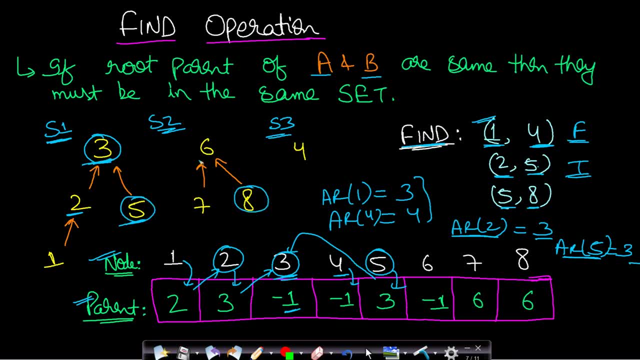 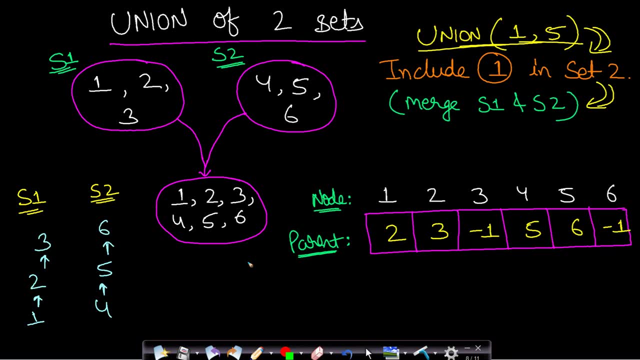 because for 5 absolute root is 3 and for 8 the absolute root is 6. therefore this will be false. so i hope you understood the find operation in the disjoint set. now the next operation is union of two sets. let us say you are having two sets, set as one and set as two. both are having three. 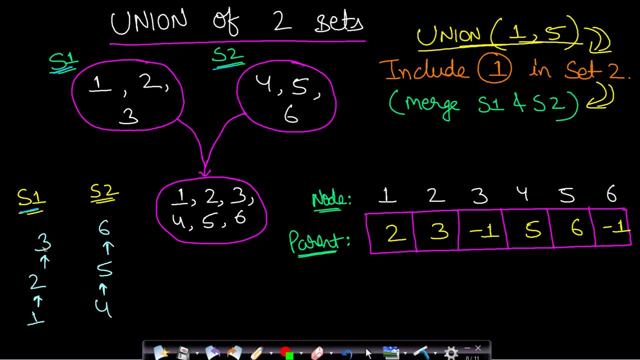 elements. now, let's say, the representation of s1 is like this: 1 is pointing to 2, 2 is pointing to 3, so 3 is the absolute root of this structure. set as 1 now. 6 is the absolute root of this structure. 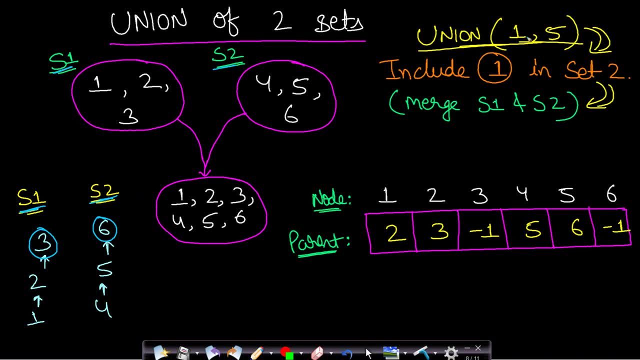 set as 2. okay, and let us assume that our operation is to take union of value 1 and value 5. that is, node 1 and node 5. so node 1 is here and node 5 is here. now how do you take the union of these two elements which are belonging to different sets? 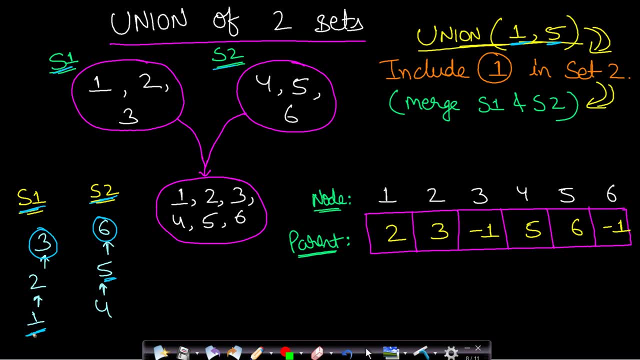 well, taking union of two elements is nothing but taking union of this one element with this set s2, and this is nothing but taking union of these two sets, which is equals to merging this set s1 with this set s2. so how do you merge it? taking union between: 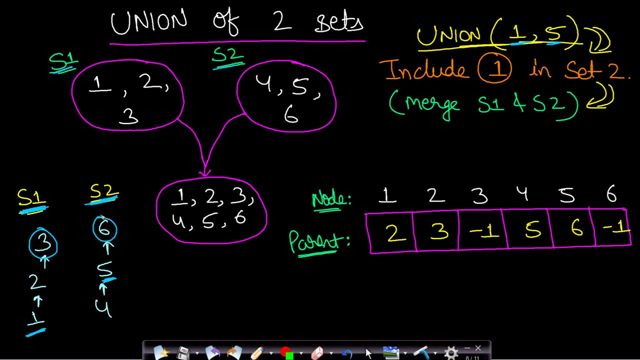 elements is basically meaning merging these two sets into one set. so what is the process for merging? well, what you can do is you can find the absolute root of this one, which is nothing but three, and you can also find the absolute root of this five, which is nothing but this six. okay, and 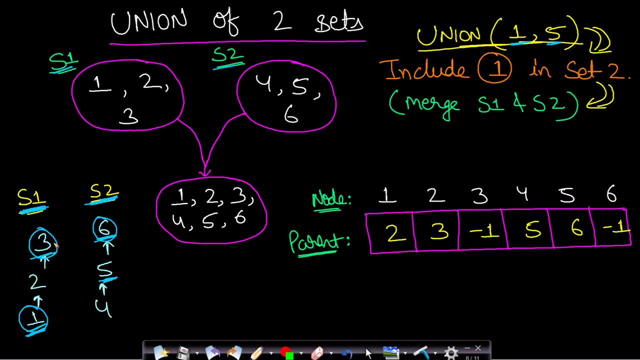 the next step is nothing, but you can make this absolute root of one point two, absolute root of five. otherwise, you can take this way as well, six to be pointing to three. both ways are correct. okay, in order to optimize it, you can take union by rank. so i will be talking about it in the further. 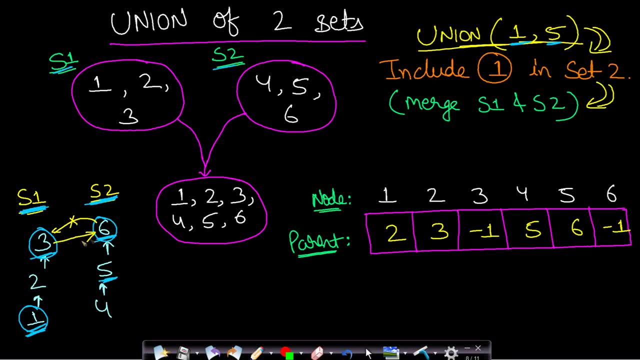 videos. so in this video i will just be sticking to the basics. in this case, let us assume that three will be pointing to six. okay, so, without pointing this, without taking the union or array, representation was like this: one was pointing to two, two was pointing to three, three was pointing to minus. 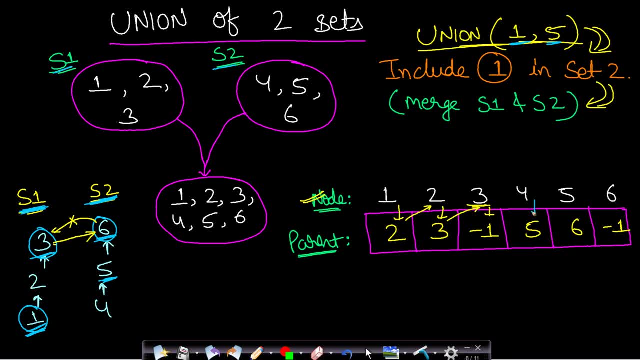 one. that means three was the absolute root and similarly, four was pointing to five, five was pointing to six was the absolute root. now we made three point to this six. okay, so how can it be done? actually, this three will be storing the value six now, so that when we reach this three then we can. 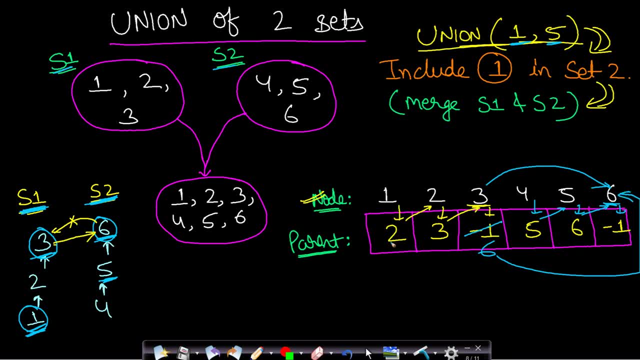 directly jump to this six. okay, so these values are actually used for jumping. that means one is pointing to two. therefore, in order to reach to this parent of one, we will simply read this value and we can jump to this index with random axis in this array. so this will just be order of one for one random axis. okay, so this is the benefit. 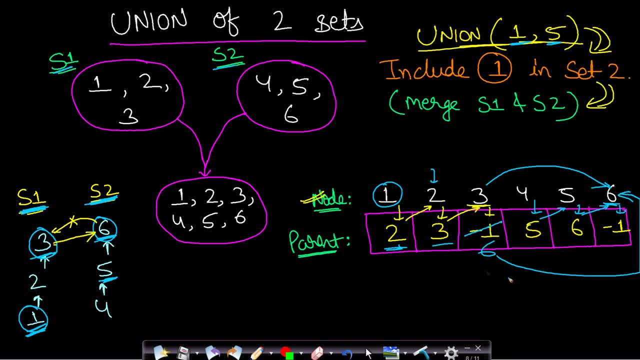 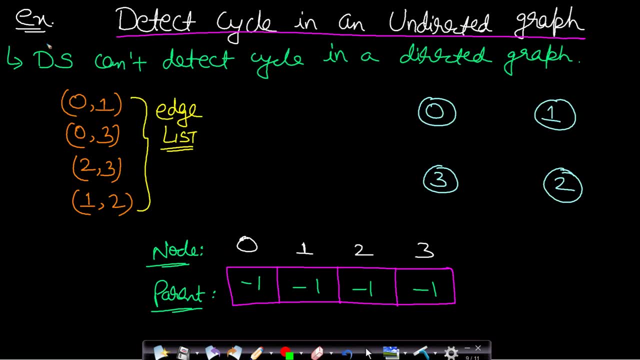 for using this array. so this is the way we will take Union of two sets. so I hope you understood this operation. now I will take a very simple example, which is to detect cycle in an undirected graph, and I will solve it by using disjoint set. so disjoint set cannot be used to detect cycle in a 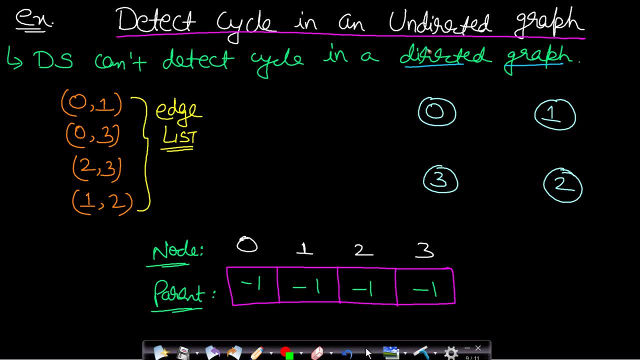 directed graph. I will explain the reason at the end of this video. first, let us see how to detect cycle in an undirected graph using disjoint set. let us assume that you are given an edge list of a graph, so in this case this is nothing but from and this: 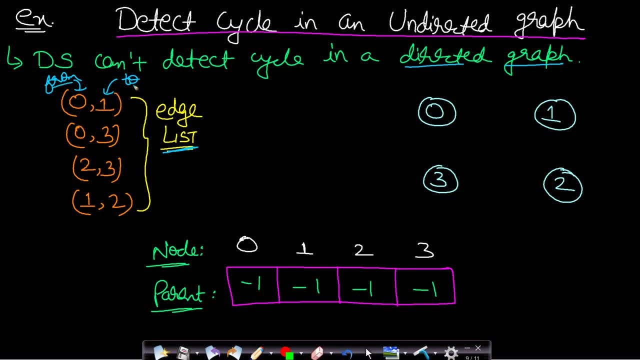 is nothing but two. and since this is an undirected graph, this from and two has no meaning because there is no directionality involved in this. but just for simplicity, I will be taking the first value as from and the second value as two. okay now, initially, we have not. 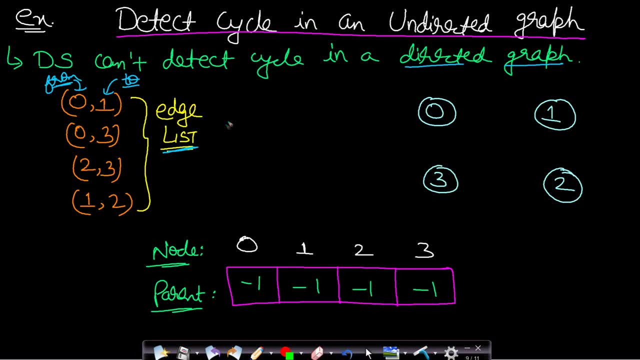 accessed any edges. and let's say we already know the number of vertices. so in this case the number of vertices are four, numbered from zero to three. so I have represented the vertices here, just for your understanding. okay, so in this case I will be taking the array for the disjoint set representation. 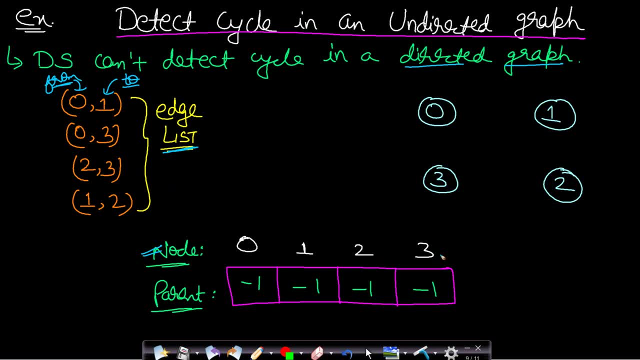 and initially all the nodes will be disjoint. that means all the nodes will be separate. they are not joined anywhere. therefore, each and every node are basically the absolute root of itself, because each and every tree is having just a single node and therefore, when all the nodes are separate, all the values will be minus one, since they are not pointing to any other node. 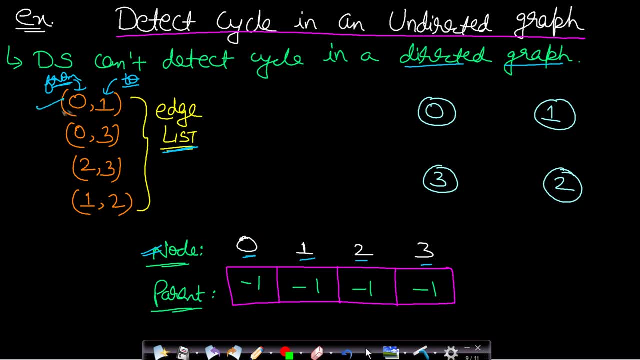 okay, now let us process the first edge. so the first stage is from zero to one. now, when the edge is from zero to one- and since this is an undirected edge, you can take either from zero to one or you can take this way as well- just for the structural representation of the disjoint set, let 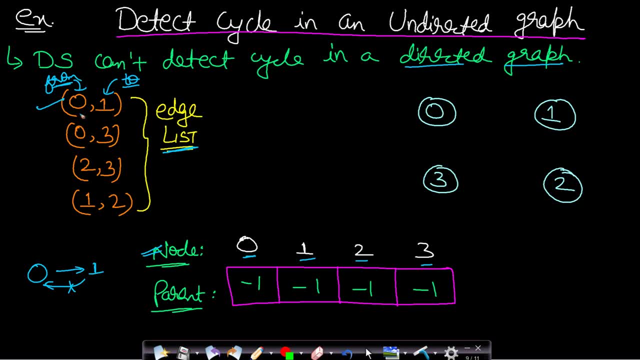 us assume that I take from zero to one. so if you take this edge zero one and you process it, then first you need to find if they both are in the same set or not. you can see that zero is storing minus one, one is storing minus one. 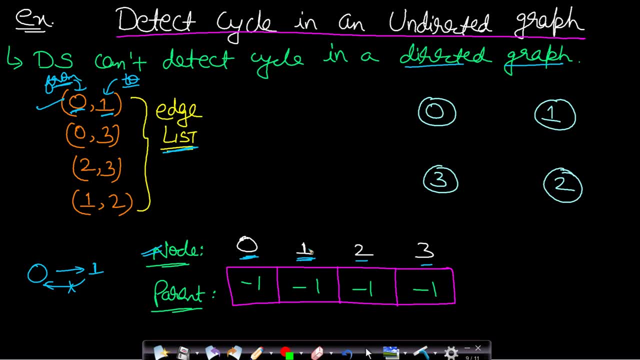 this indicates that zero is the absolute root and one is also the absolute root and since they both are having different absolute roots, therefore they must be in a different sets. okay, so we can take Union of them. so taking Union of them is nothing but pointing one absolute root to another, as I have already explained you here when we had taken Union, then 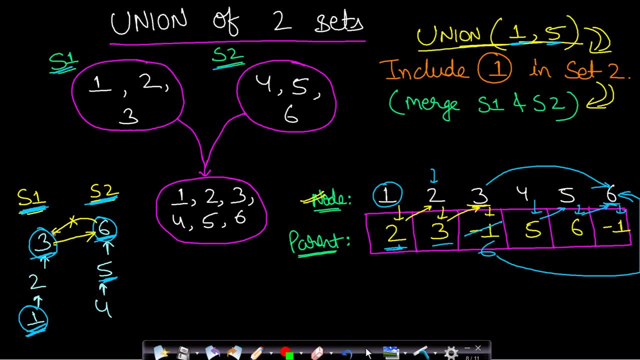 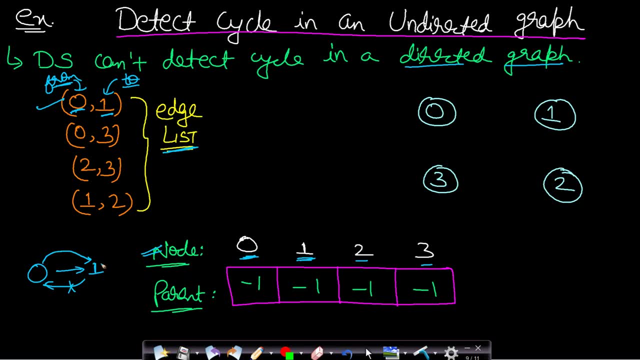 three was pointing to six, or you could have made six pointing to three, okay, so in this case I will assume that I will take this zero pointing to one. so when zero is pointing to one, then one will become parent of zero. so you will have to replace the value for zero, and this will now be equals to: 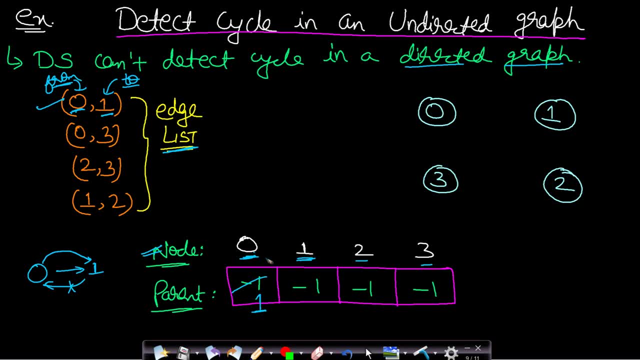 one. this will represent that zero and one are in the same set and zero's parent is one, and one will be absolute root, since it is storing value minus one. so this edge has now been processed, and so we will, let's say, add them. okay, now we will process the second edge, which is from zero to three. so 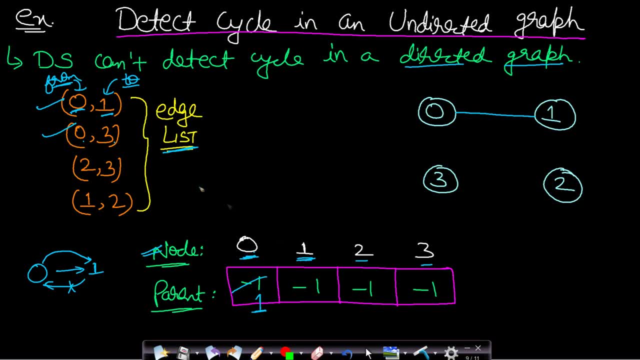 what is the absolute root of this zero? absolute root of zero is one, and absolute root of three is three itself. therefore, zero and three are having different absolute roots, and so they must be in different sets. so what we will do is we will take Union of zero and three, so zero's absolute parent. 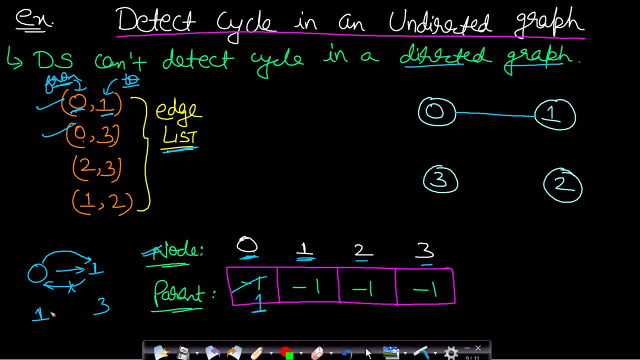 three's absolute parent is three. so taking Union of one and three is nothing but pointing one to three. or you can take pointing three to one, but I will take, let's say, from one to three, so one will now be pointing to three. therefore, the value stored here will now be updated to three. okay, 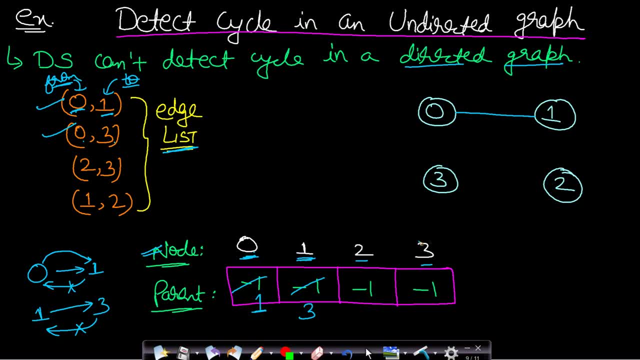 so one will now be pointing to three. so zero, one and three are belonging to the same set now. so we will draw an edge here. okay, now let us process the third edge. so the third edge is from two to three. so we will find the absolute root of this two, absolute root of this three, absolute root of two. 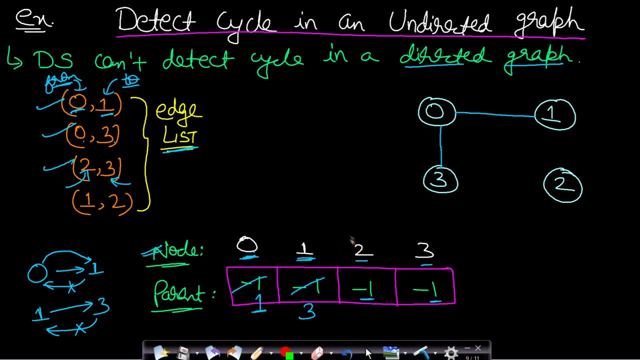 is two itself. absolute root of three is three itself. so what can we do? we have these two absolute roots as different, therefore they must be belonging to different sets, so we can simply join them, and by joining I mean we will take Union of them. so if you take Union of two and three, then 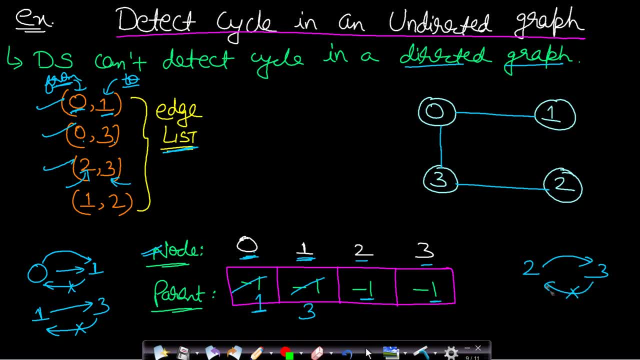 this means you will be pointing two to three or three to two. I will take pointing two to three, so I will update your value two to three. okay, now we have processed first three edges and you can see that there is no cycle. so we were not able to find any cycle here. but as soon as you add this fourth, 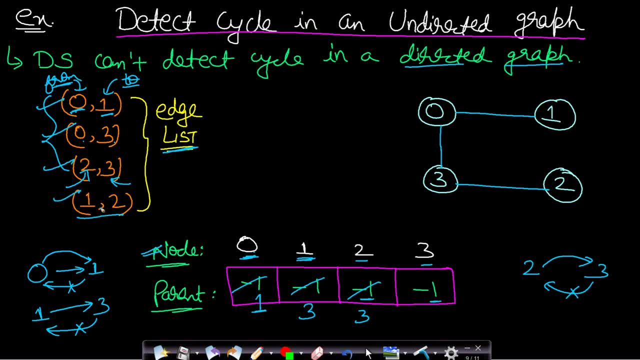 edge, then you will find a cycle. let's see, you want to add this edge one comma two. now the absolute root of this one is equals to three. okay, because from one you will jump to three, and three is having value minus one. absolute root of this two is also three, because from 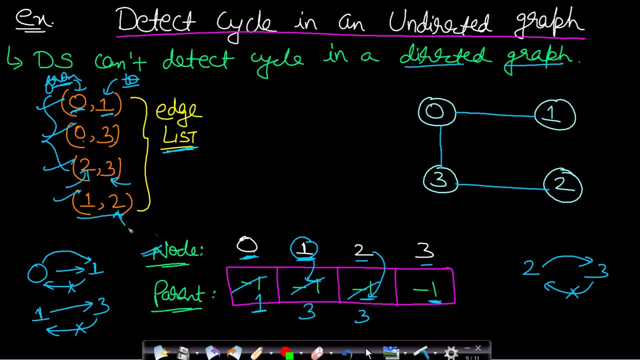 two you will jump to three and from three you will have minus one. so absolute root of both these values, one and two are both threes. so since they are having both same absolute roots, therefore they must be belonging to the same set. that means we will be having a path from one to two in. 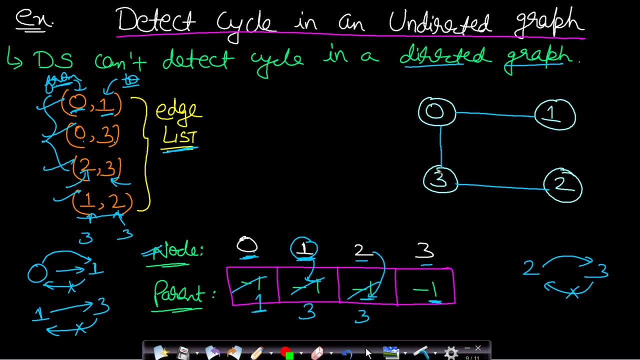 this case, you can see that there is a path from one to two via zero and three. okay, so they both belong to the same set. now, if you add this edge- that is, an extra edge between two elements are belonging to the same set, then this will obviously create a cycle. okay, this is very. 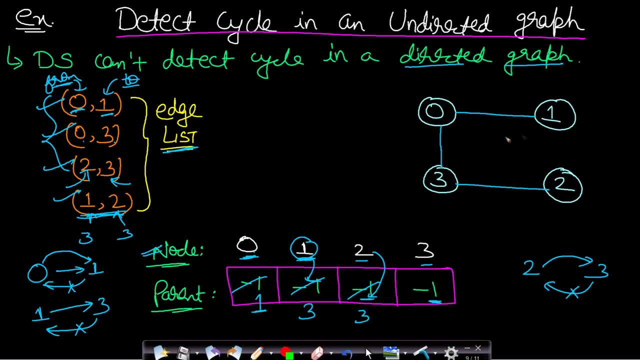 obvious. think about it: if one and two are belonging to the same set, that means they are already having a path between one and two. and if you want to create a direct path, which will be an alternate path between one and two, then that will obviously create a cycle, because there was already a path. 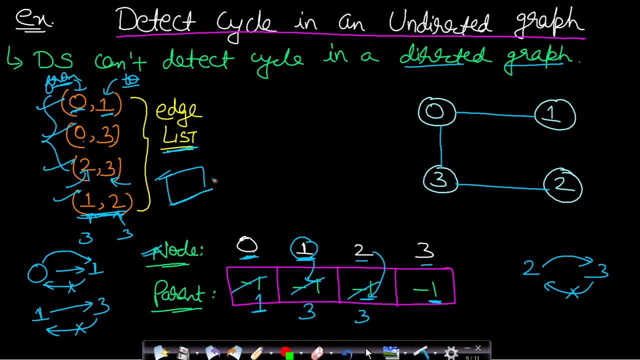 and you are now connecting them both directly using another path, so this will definitely create a cycle. so in this case, they both are having same absolute parent values. therefore, we will simply return true, saying that adding this edge will create a cycle. okay, so this is the way in which a disjoint set can be used to. 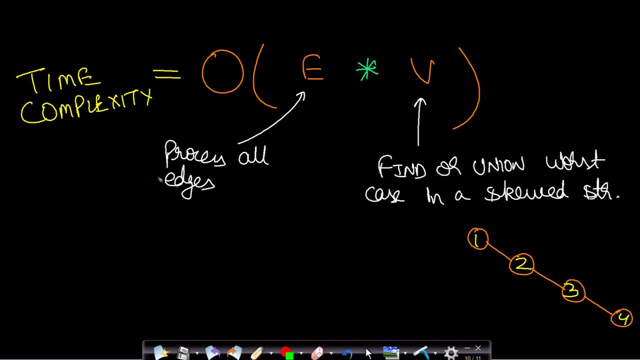 detect cycle in an undirected graph. now, what will be the time complexity? well, the time complexity will be order of E into order of V, because we are processing each and every edge from the edge list one by one, and this V is for traversal, for the second operation, in order to find the absolute root, because you can have a skewed tree and 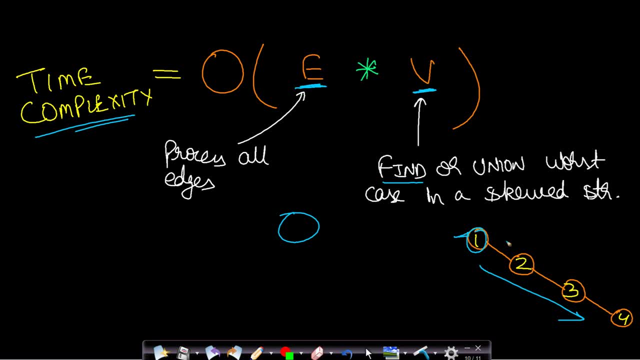 whenever we add like, we have this one as the absolute root. when we add this two, then we will find the absolute root. when we add this three, then we will also find the absolute root by jumping, like this. and when we add this four, then we will also find the absolute root by jumping. so in this. 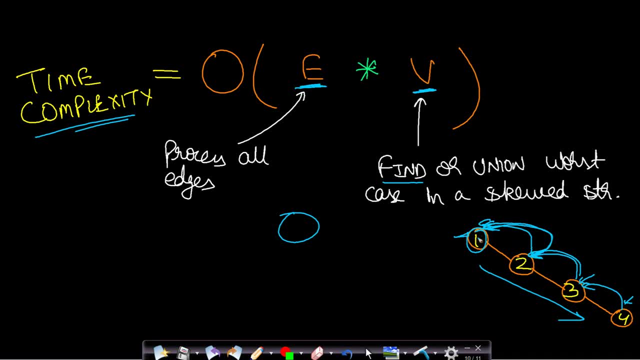 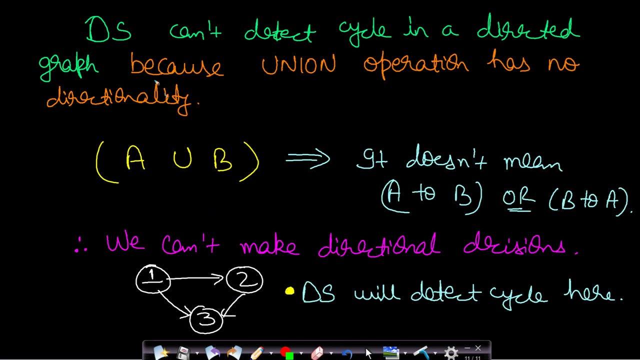 case. this is nothing, but we can jump V times in worst case. so for each edge addition you can jump the maximum of V number of times. so the total time complexity will be E into V. this will be much more clear from the code. so before seeing the code, I will explain you the reason. disjoint set can't. 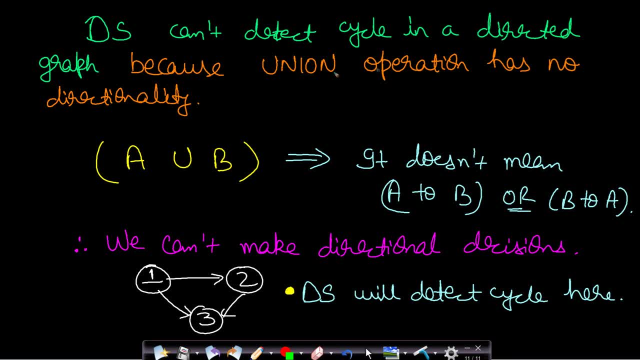 detect cycle in a directed graph, because Union operation has no directionality. if you take a Union B, then it doesn't mean A to B or from B to A. it has no directional meaning. therefore we cannot take directional decisions. let us say: if you take this graph, 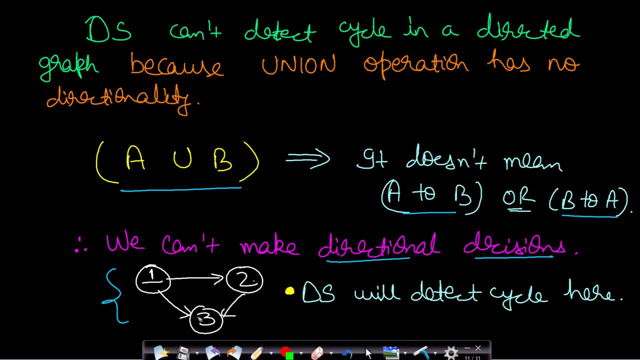 one pointing to two, two pointing to three and one pointing to three. in this case, you can see that there is no cycle, but if you use the disjoint set data structure, like I have already explained, then this will detect a cycle. okay, try this and you will get a better understanding. now let us look. 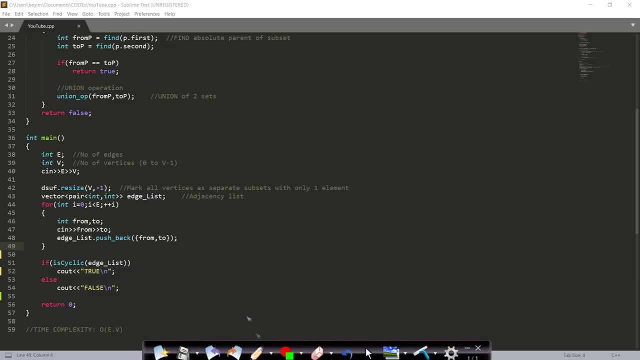 at the code. so this is the code which I have written. in this case I will take the input as number of edges and the second input as number of vertices. so this is E and V, and I have also taken a array which I had already represented. index will be representing the node. 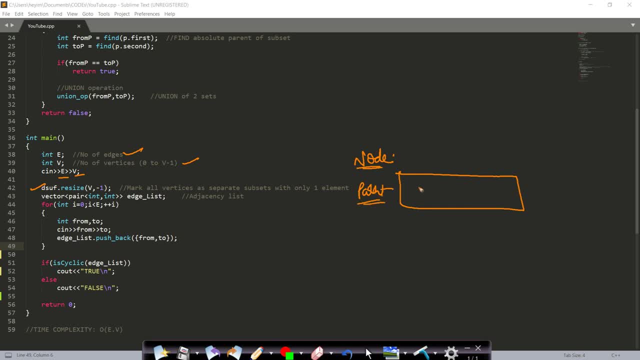 value and the value will actually be representing the parent. okay, so this: I have named it as dsuf as disjoint set Union find operations, so you can also name it as parent. this is a more meaningful name, but I have named it as dsuf. now, after taking the edges and vertices as input, I will take the edge. 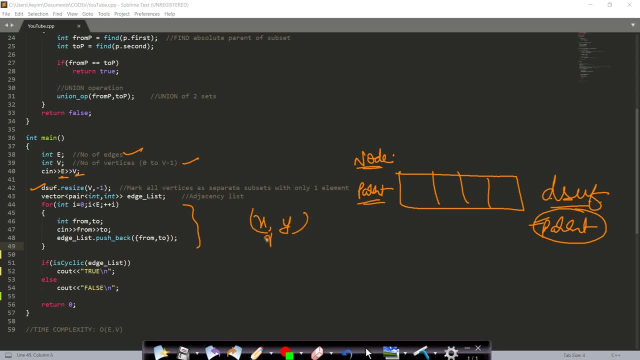 list. so the edge list will be having x, comma y, which is nothing but from, and this will be two. okay, and I will keep inserting all the edges in the edge list. after preparing the edge list, what we need to do is we need to simply find if there is a cycle. if there is a cycle, then I will print true, otherwise I will. 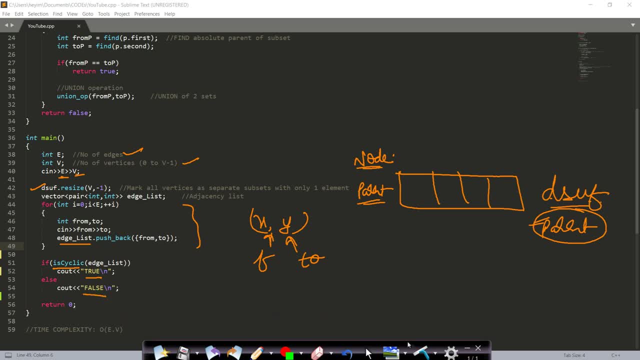 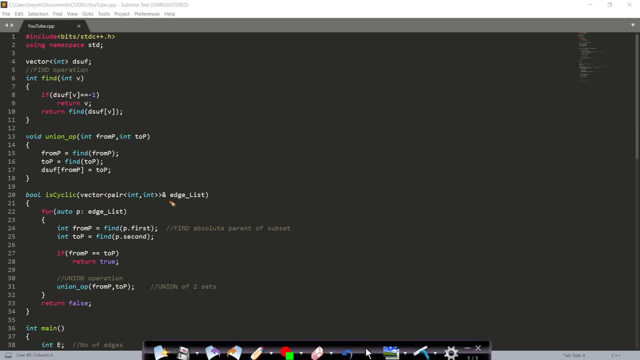 print false and then we will end this entire program. so let us now see the cycle finding algorithm. in this case, you can see that I am receiving the edge list and from this edge list I will pick one edge pair one by one. so edge list will be having pairs of. 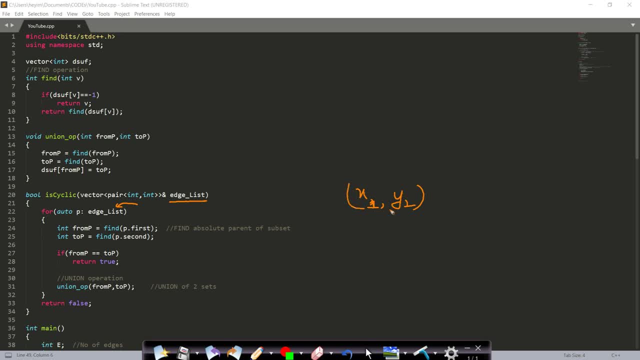 to and from. okay, so this first one is from and the second one is two. as I have already explained you, this will be x2, comma, y2 and so on, so these will all be in pairs. so I will take each and every pair one by one. so this P is a pair, P dot first means the first element, that is, from, and P dot second. 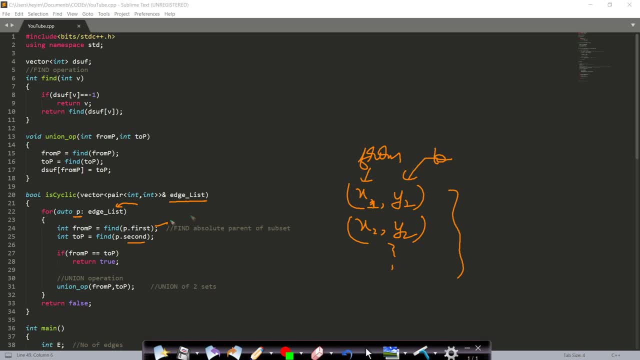 means the second element, which is nothing but two. okay, now, when we take both these elements, the first one and the second one, then I will find the absolute parent of this first value and the absolute parent of the second value. if the absolute parent of first and second are same, then this will indicate that they both are already present. 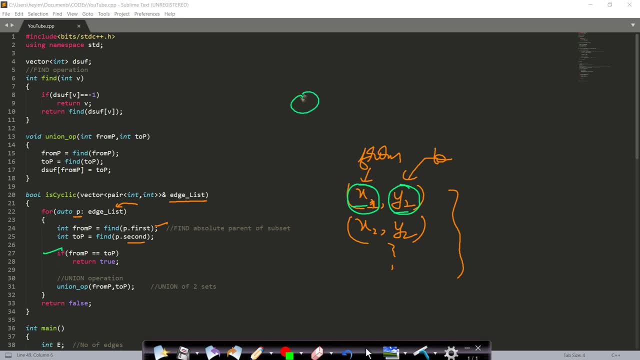 in the same set and since they are already present in the same set, this will indicate that there must be a path between them, and if we are willing to join them directly, then this will obviously create cycle, and since adding this age will create a cycle, therefore we will have to return true. 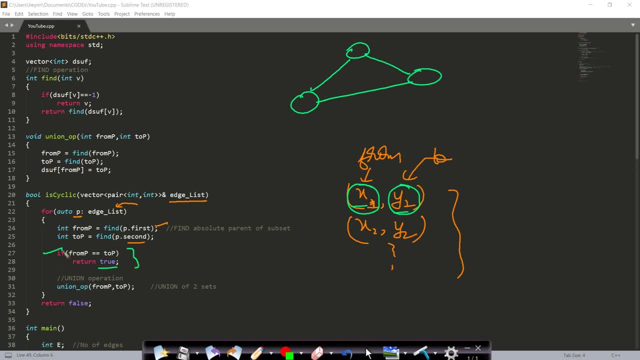 saying that adding this age will create a cycle. now, if the absolute parent values of from and to are not the same, then we will simply join them by using union operation. so let us see the find and union operation. so the first operation is for finding the absolute parent. this will be nothing. 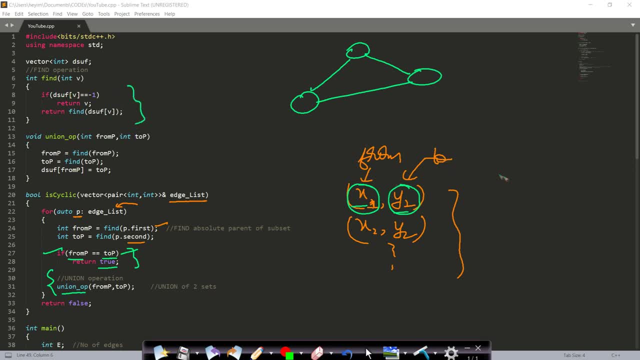 but a recursive method in this case. this is a very simple method. let's say you are having a value 1 pointing to value 2, pointing to value 3. okay, so in the array representation what you will be having is you will be having like this: so 1 will be pointing to 2, 2 will be pointing to 3 and 3 will. 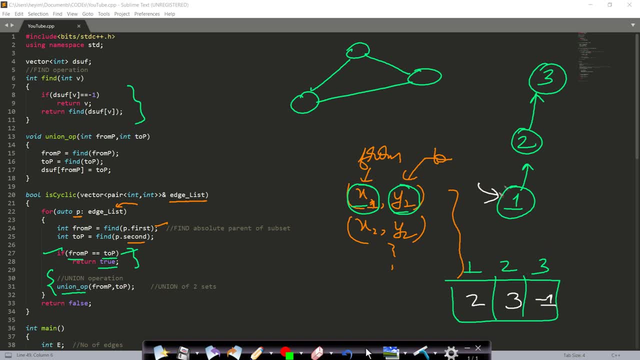 be having value minus 1. now, if you are at this 1 and let's say the value at 1 is 2, then you will go to this 2. value of 2 is 3. you will go to this 3. now value of 3 is minus 1. so as soon as you hit, 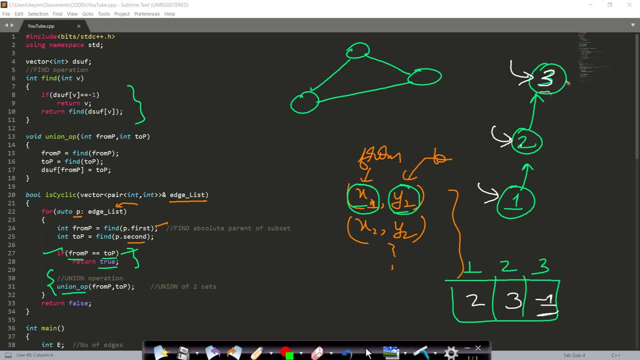 a node with a value minus 1, then that node must be the absolute root of your node, which you wanted to find. therefore, you will simply return this node, value 3. in this case, you can see that the recursive formula follows the same approach. in this case, if you are at a value, let's say at vertex v, and that is storing value, 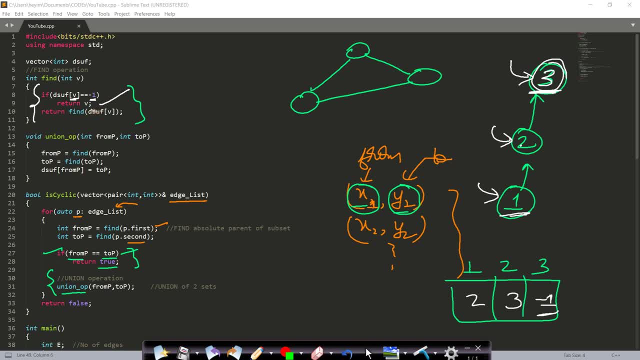 minus 1. this indicates that vertex v is the absolute root, and you will return that vertex. otherwise, if it is not storing minus 1, then that is an internal or a leaf node, and so you will be also used in that way. you can also use this find at v as well, so you can also add a unique find at. 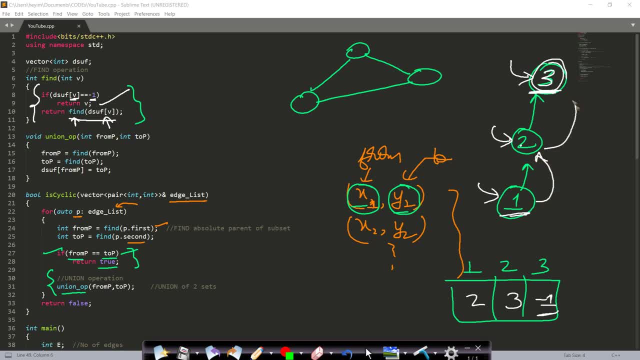 v. let's say, after this find at v, you will call the find operation on its parent. so you will again call the find operation on its parent. so dsuf at v is nothing but the parent of v. okay, so in this way you will recursively jump one level at a time unless and until you hit the absolute root node. 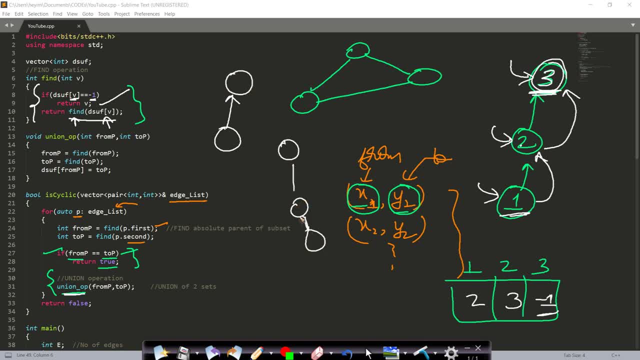 okay, so this is the find operation. now, after this find operation, you will see this union operation. you want to find the union of these two? then you will find the absolute root of this node x and absolute root of this node y. so now you will call the union for these two node values, which is from: